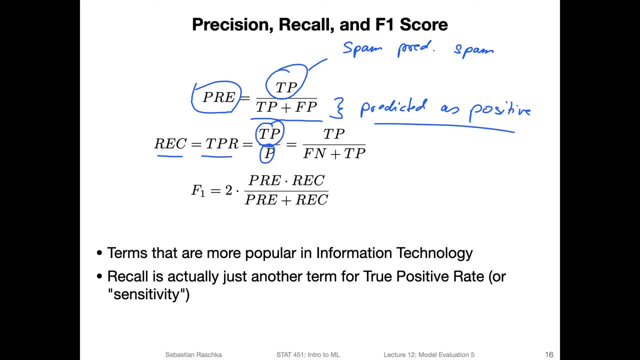 do we actually recall? so the true positives are the ones that we correctly predict as positive. So how many out of the positives do we actually identify as positive? It's like, how are we doing on recall? How many do we actually identify as positives, given all the positives and a 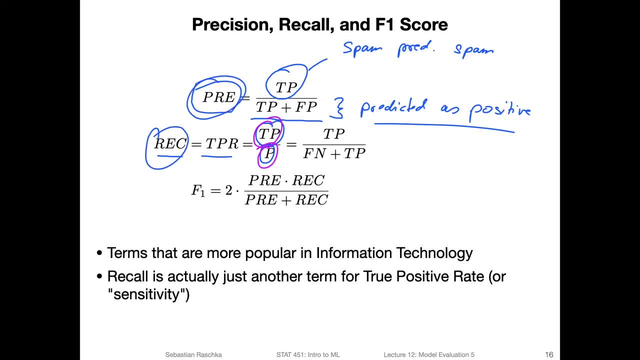 weighted version of the two of precision and recall is the so called F one score. So the F one score, you can think of it as a combined version of precision and recall, which is using both and then multiplying it by two. So the range of all these 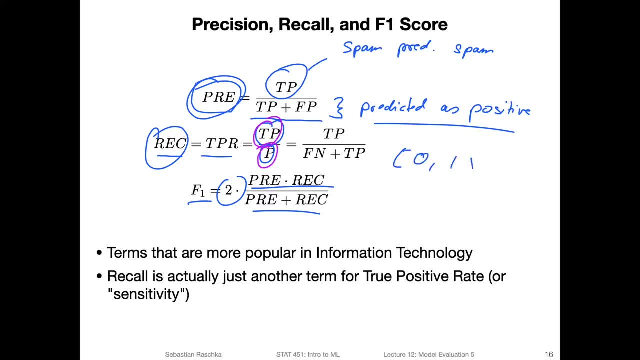 metrics is between zero and one. So I'm writing here. I see in my notes that terms that are more popular, So these are terms that are more popular in information technology. By that I mean there are other terms called sensitivity and specificity. sensitivity and specificity are terms that are I. 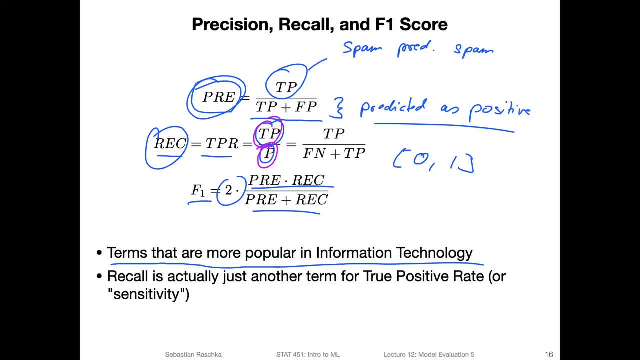 would say more popular in computational biology, for example, whereas precision and recall are terms that are more common in information technology technology or computer science and machine learning. So if you would write a paper, for example for a computational biology journal, using machine learning, then maybe using 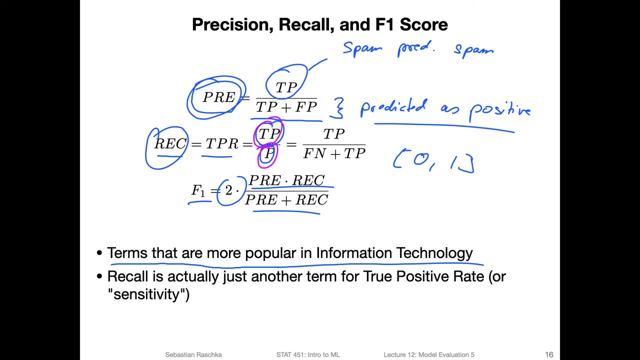 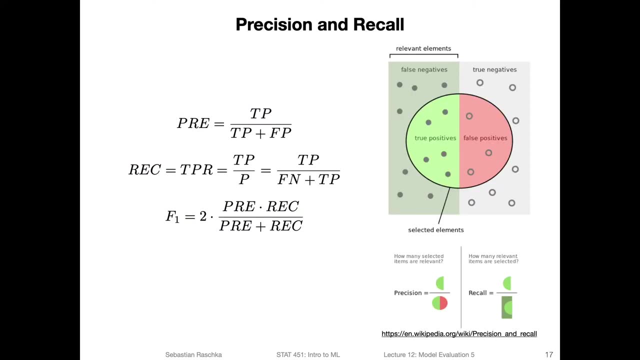 precision and recall is not the best idea, because most people in computational biology use sensitivity and specificity to analyze their systems. So, yeah, like I said, recall is actually just another term for the true positive rate. Yeah, here's a helpful visualization of the precision and recall that I took. 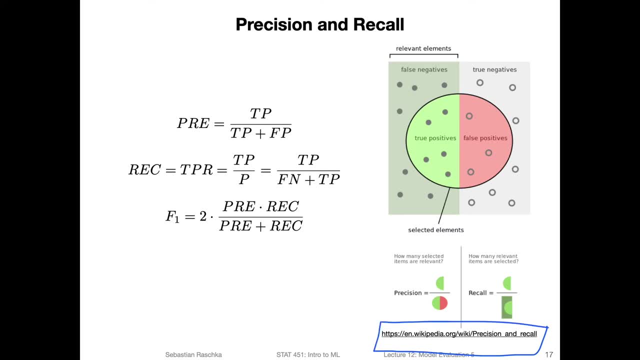 from Wikipedia. I kind of like this visualization because it's just easy to see what's going on. So you can think of everything here on the left- the left box- as the positives in the case of spam classification, the spam email- and these as the negative class. 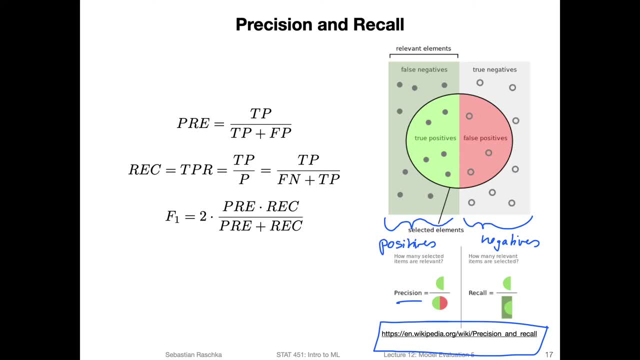 And then the precision is computed as the fraction of the true positives. So that's the true positives over all the predicted ones. So these are all the ones that are predicted as positive. So that's the fraction of the actual positives, the true positives predicted as positives, over all the ones. 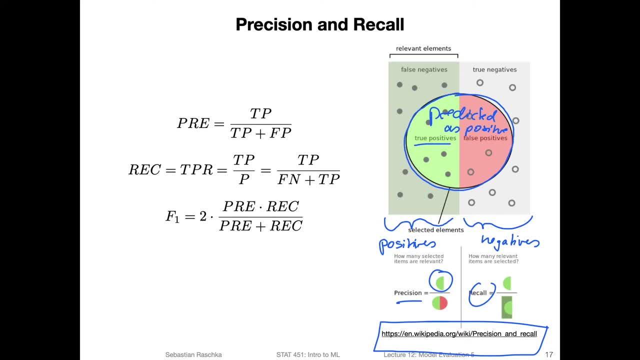 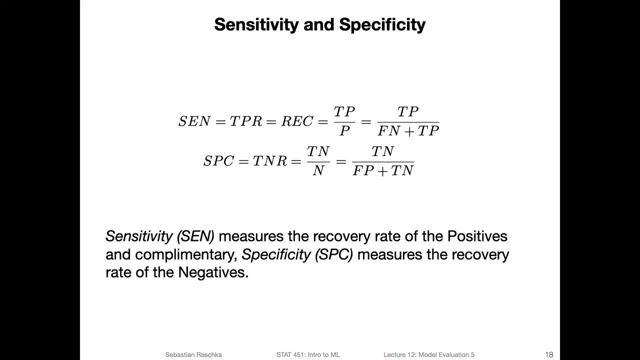 predicted as positive, whereas the recall gives us the number of true positives over all the positives, for instance. So he has just a helpful visualization of this metric, of the precision and the recall. recall. Now, um yeah, like I said, there are two. 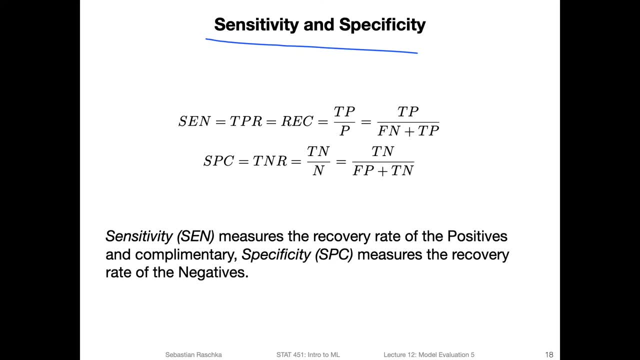 other metrics that are commonly used, for example in computational biology. it may also be common in other fields. I just I didn't work in many other fields except machine learning and computational biology. I know for a fact: in computational biology, when you talk to biologists, most of them 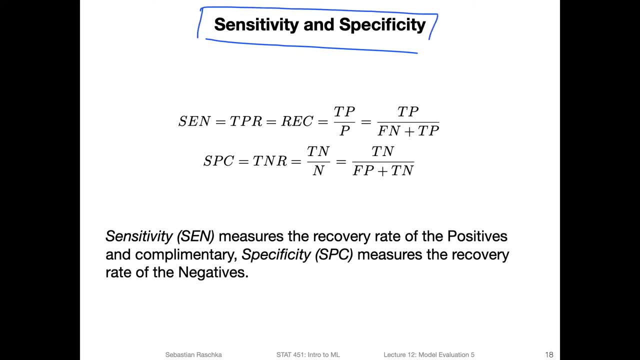 are familiar with sensitivity and specificity. However, in computer science, if you mention sensitivity and specificity to someone or most people don't know what that is. most people are familiar, though, with precision and recall. In any case, sensitivity is just the same as 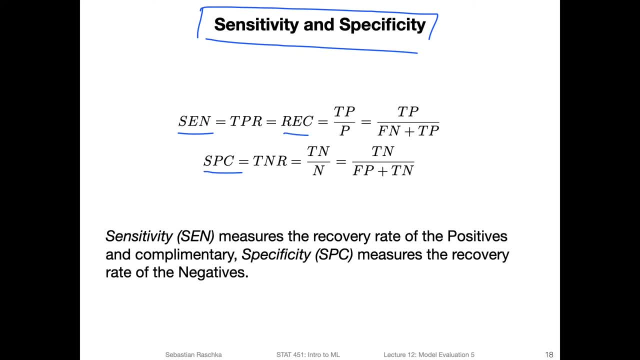 recall, it's just another word for recall. specificity is a little bit different. It's the number of true negatives over the number of negatives, So it's kind of the opposite of sensitivity. I think it's kind of intuitive yet to remember it. 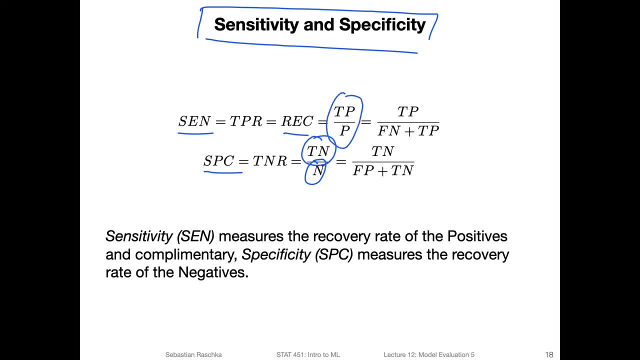 like this, because here you have the true positives over the positives And, for specificity, you do the same thing except for the negatives, the true negatives over the actual negatives. Alright, so it's some. sometimes people also say it measures the recovery rate of the negatives, whereas the 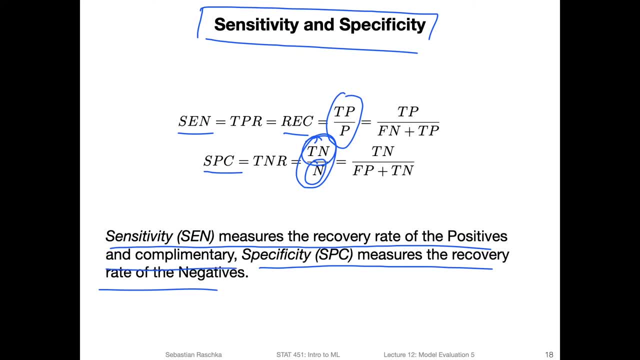 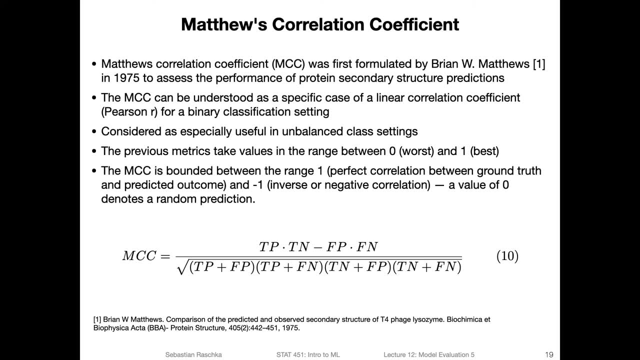 sensitivity measures, the recovery, recovery rate of the positives, Okay. so, lastly, there's one more thing, that's Matthews correlation coefficient, And this is also something that is commonly used in the context of biology, originally for assessing the performance of protein: secondary structure predictions. So what is a protein? 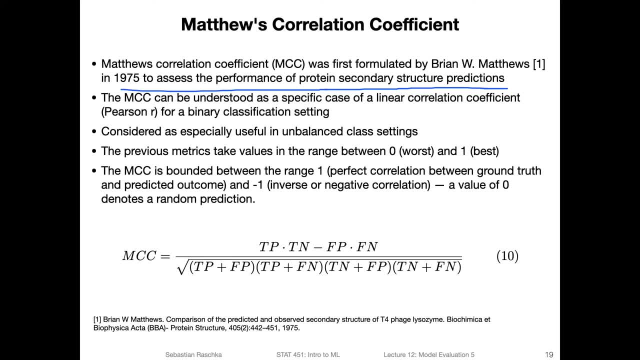 secondary structure prediction. So if you think about amino acid sequence, so where you have an amino acid sequence like as follows: it's not a DNA sequence, it's an amino acid sequence- And then from that, from the sequence, you can 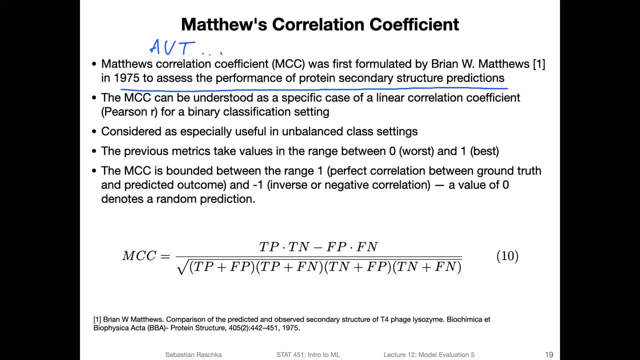 predict whether a subsequence is in the 3d structure, for example in an alpha helix on a beta sheet, and so forth. So you're predicting alpha helices, which are three dimensional structures based on the sequences. So in that way, yeah, there are algorithms to. 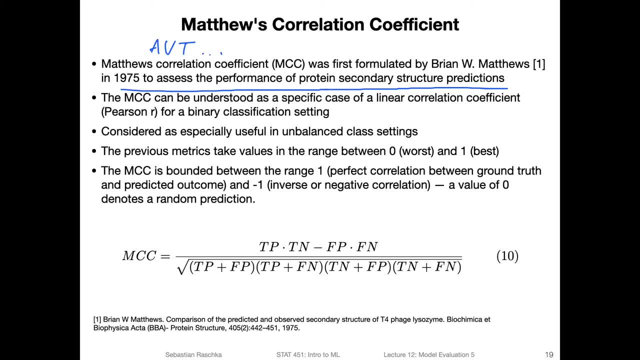 predict that. And, Matthews, correlation coefficient was back then formulated to assess the performance of these prediction algorithms. So you can think of it as a version of linear correlation coefficient, But instead of like a Pearson's r for linear regression, you would have that for a binary. 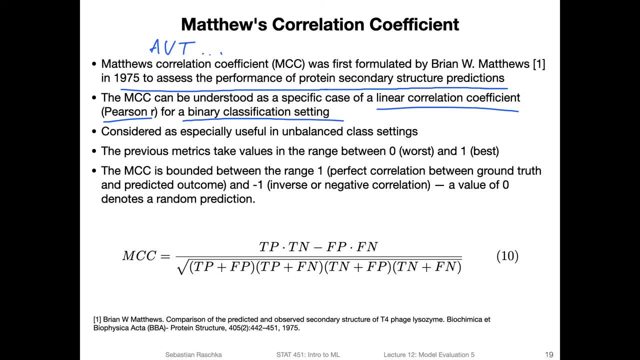 classification setting. So it's. it's like a, yeah, like a correlation coefficient for classification settings And sometimes also it's often regarded as useful in imbalanced class problems, where you have a problem where one class has more examples than the other. So in some cases I see 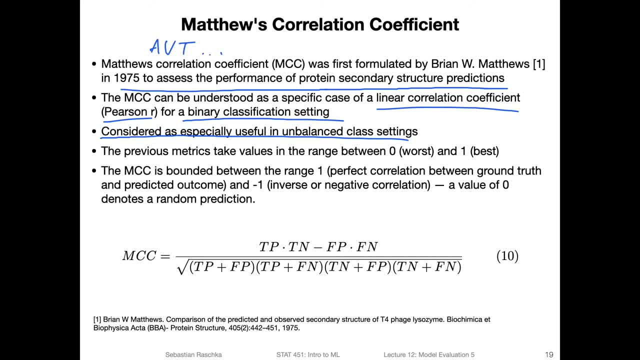 that also recommended for imbalanced class problems. So the previous metrics that we talked about, specificity, sensitivity, recall precision if one score and so forth. they were ranging between the values zero and one, where one was best. So measured Matthews correlation coefficient. now, 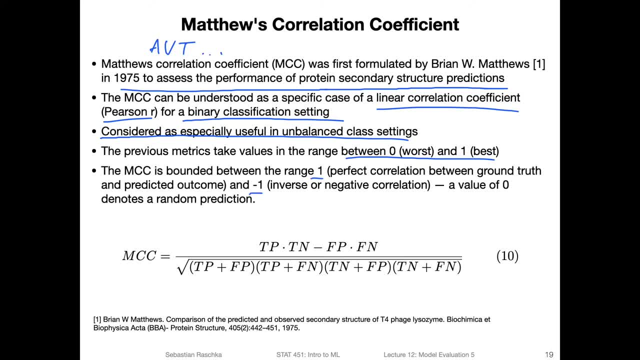 ranges from minus one to one, similar to your Pearson's r correlation correlation coefficient. So Pearson's r also ranges between minus one and one. Wherefore, if you recall Pearson's r, if you have minus one, you have a negative correlation. for zero there's no correlation And for one there's. 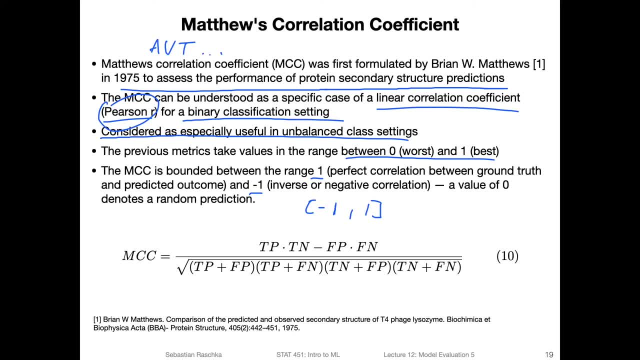 a perfect correlation. And analogously for Matthews correlation coefficient: you have a perfect correlation if you have one. So that means that you have a perfect match between the actual ground truth label, so the true label and the predicted label. And if you have them completely flipped, if you 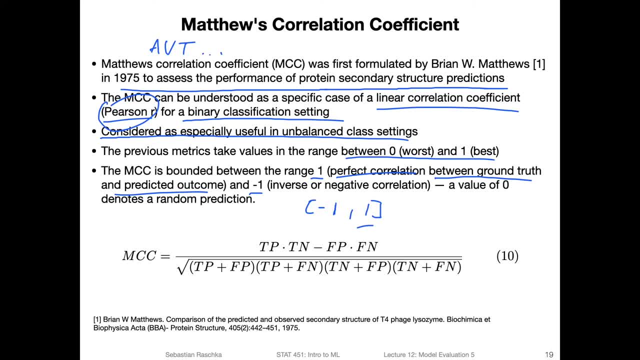 predict everything, every positive as negative and every negative class as positive, then the correlation coefficient would be minus one, And if the prediction is completely random, then you have a value of zero. I think it's kind of intuitive and useful also in practice, just to see how your classifier performs. So 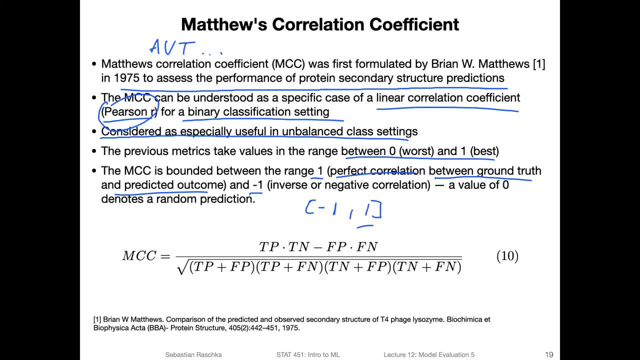 for example, if you see that your classifier has a minus one in terms of the Matthews correlation coefficient, it might be just useful to flip the predictions, and then you have a perfect classifier. Okay, so yeah, that's Matthews correlation coefficient. Here are, lastly, some code examples for the: 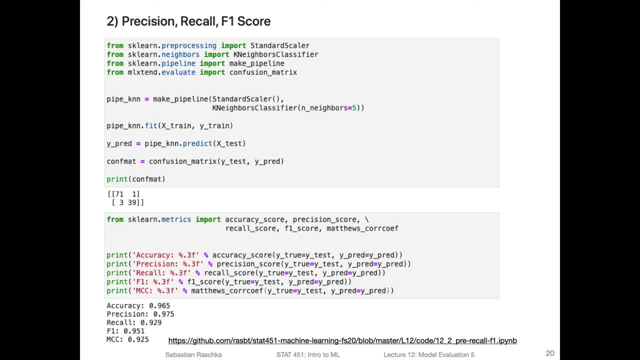 different metrics that we talked about. So here's just again what we had before: our k nearest neighbor classifier, together with a standard scale up on the Wisconsin breast cancer data set, And this is the confusion matrix that we had. And then we don't actually need to use the confusion matrix, is just for. 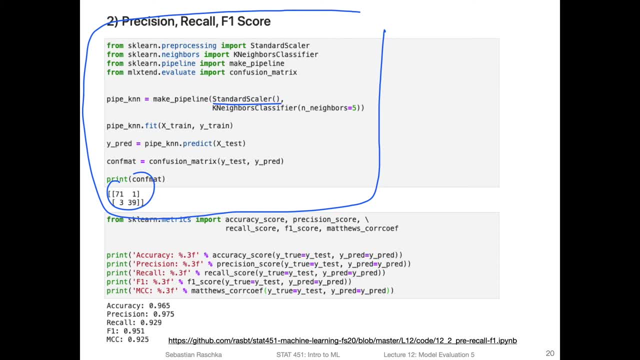 reference. we can import the scores like the precision score, recall score of one score and Matthews correlation coefficient from psychic learn, Yeah, just apply them to the test labels versus the predicted level labels and get different metrics. That's how you can use it. So you could technically also just compute that from the 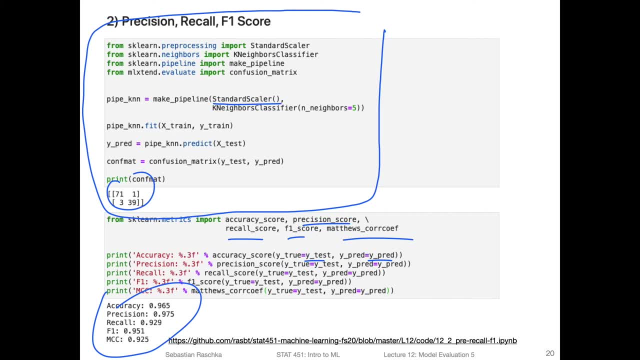 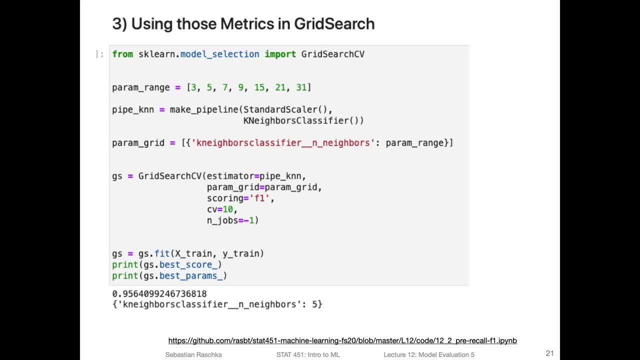 confusion matrix. But yeah, that's not necessary, So we can also use these metrics in grid search. So instead of providing, for example, these function as input, you can also use a string, for example F one, four, F one score, or the string. 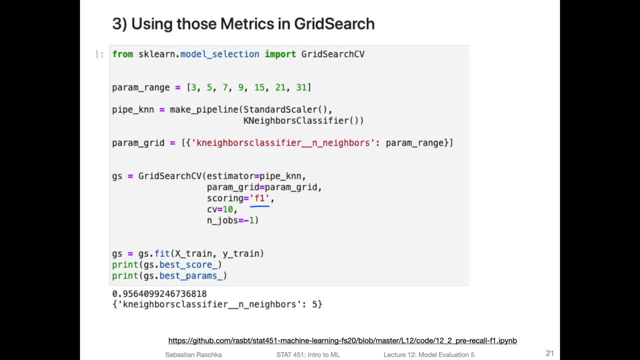 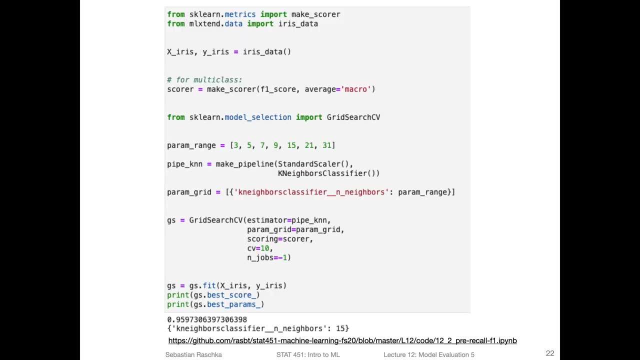 precision for precision and then do grid search and hyper parameter tuning with these metrics instead of using the classification accuracy. Note that for multi class problems it's a little bit trickier because all these metrics we discussed so far are binary metrics, So they only work if 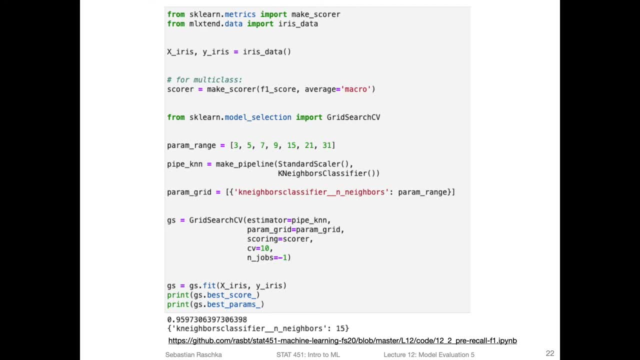 you have two classes like zero and one. So if you want to use, for example, precision, recall or the one score for multi class, then you have to do a little workaround. So you would use the make score function and then make a score using, for example, that one score and set. 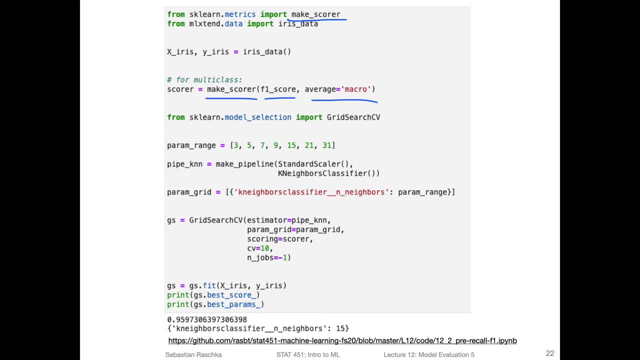 the averaging to micro or macro. we will talk more about micro and macro in the last video in this lecture. But yeah, if you want to do that, then here. I mean if you are basically trying to do a multi class problem, and it doesn't work. 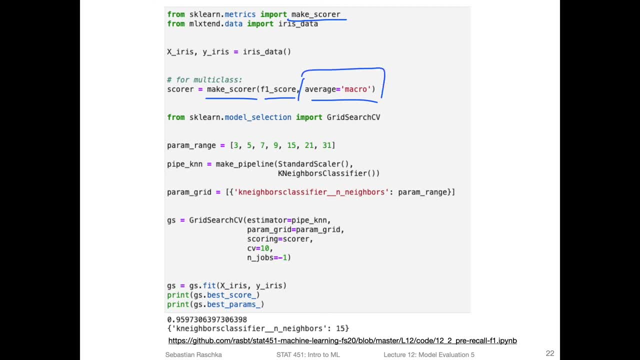 using F one score, then you know it's because you probably didn't do the average, And what that means will be that you can do it with the standard metric, for example. you can do it with the standard metric, or you can do it with. 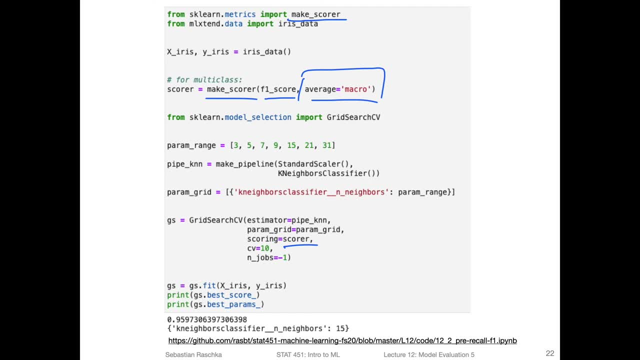 the standard metric, or you can do it with the standard metric and then you can do it with the standard metric. So that's something that we discussed in the last video. And, yeah, we can then provide the score also to the grid search, And this is how. 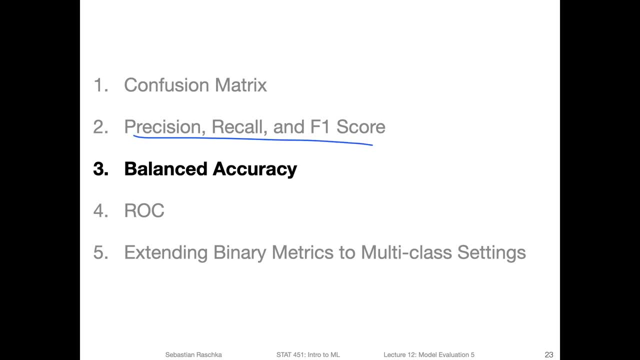 we can use different metrics instead of just classification accuracy to do the grid search. Okay, that was probably more of the boring videos because we just went over some additional metrics. In the next video, I will talk about balanced accuracy, and this is also then for can be used for multi class actually. 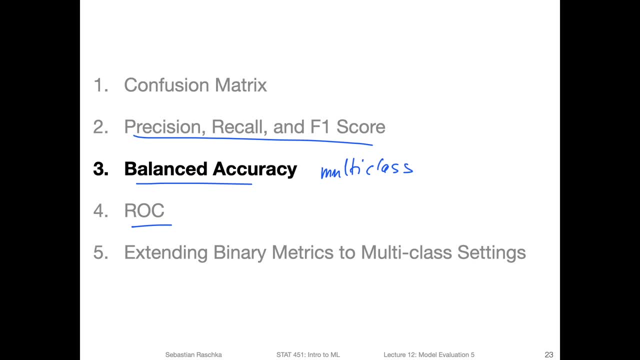 So this will be also interesting. And then we will talk about receiver operating correct characteristic curves and then extend the binary metrics to multi class settings. Okay, so I will see you in the next video. 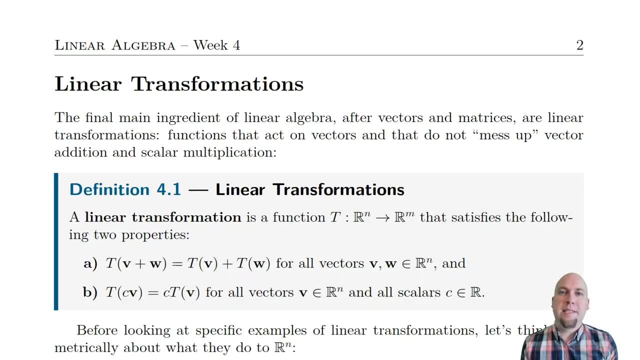 Hey folks, my name is Nathan Johnston and welcome to Lecture 13 of Introductory Linear Algebra. Today we're going to start learning about something called linear transformations, And what these are is they're functions that send vectors to vectors. So, for example, 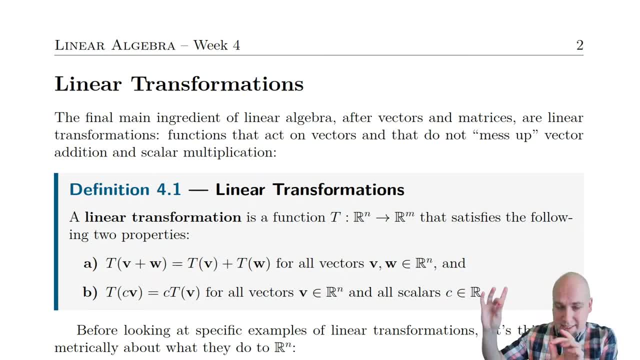 if you've got a vector with two entries, then a linear transformation just takes that vector with two entries and moves it somewhere else, So it spits out some other vector. So it's got your vectors as inputs and that gives you vectors as outputs And I mean it might send a two. 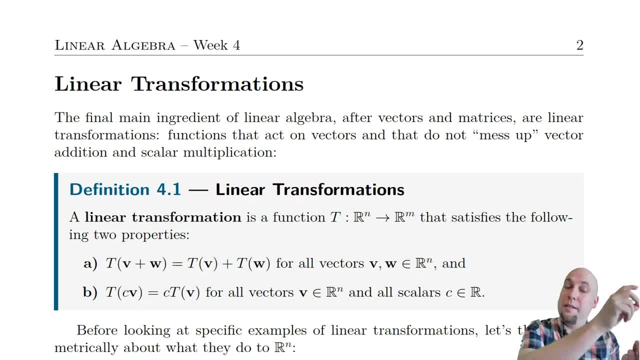 dimensional vector to a two dimensional vector, might send a three dimensional vector to a three dimensional vector, or it might mix and match dimensions as well, Like it can send a two dimensional vector to a seven dimensional vector. Okay, but it turns out that studying all functions 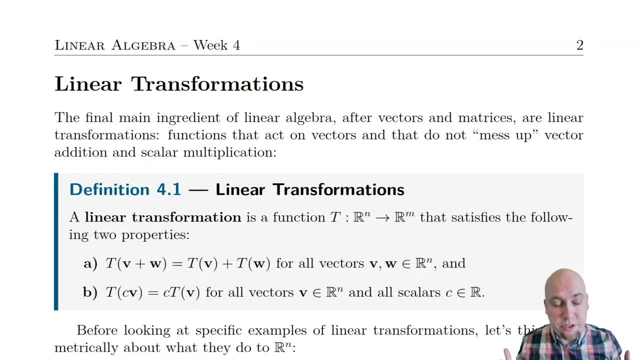 that send vectors to vectors is too complicated, Okay. there's just no hope of having nice theorems that say: ah well, if you've got a function that sends vectors to vectors, then this happens. It's just too wild of a set, Okay. so what we do is we restrict our attention to functions that. 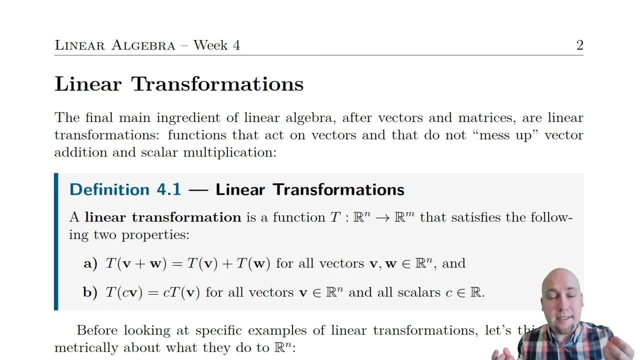 send vectors to vectors, but do so in a way that we don't want to. So what we do is we restrict our attention to functions that send vectors to vectors, but do so in a nice way. They have to send vectors to vectors in a way that basically plays well with other linear algebra things.